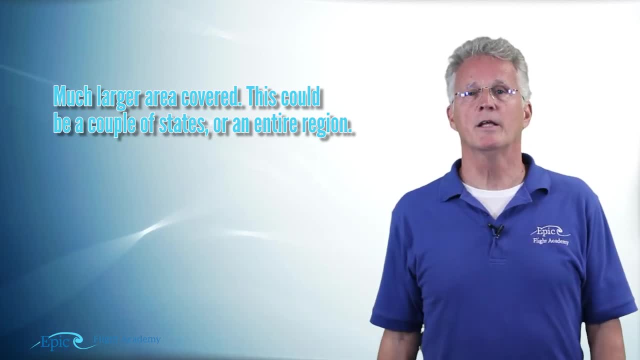 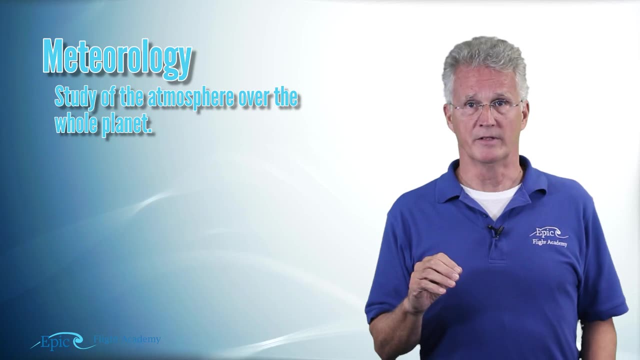 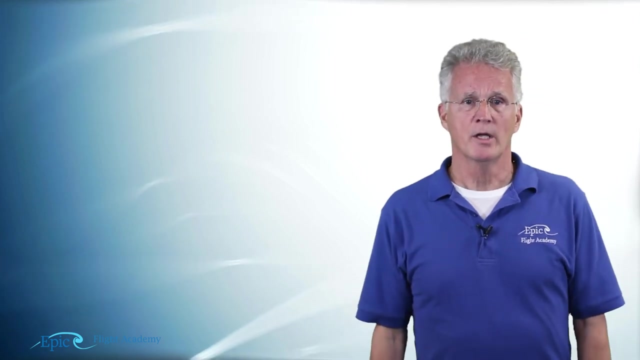 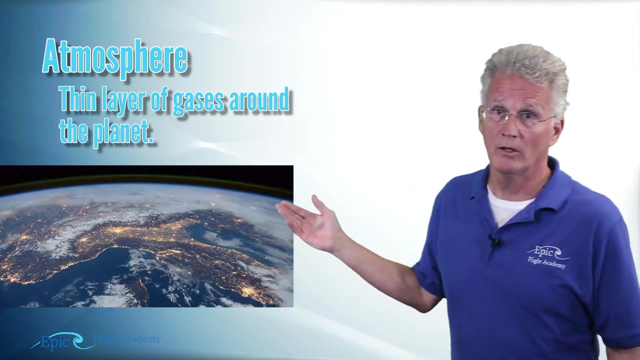 might be spoken of as a tropical climate. And then, finally, meteorology. Meteorology is a science. It is the study of the atmosphere around the entire planet. The atmosphere of planet Earth is a thin layer of gases. It surrounds the entire Earth And you can see here- this is a picture from a satellite- 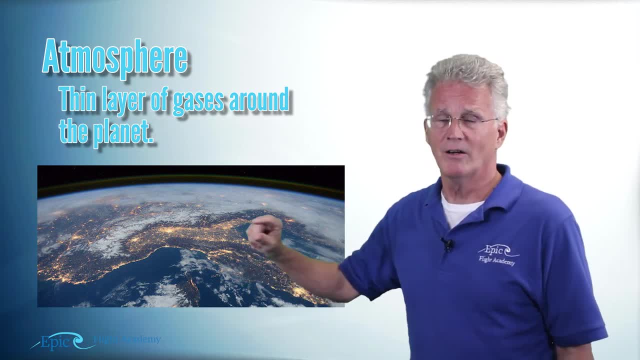 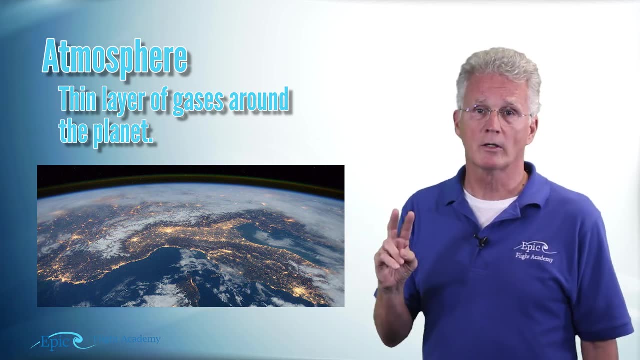 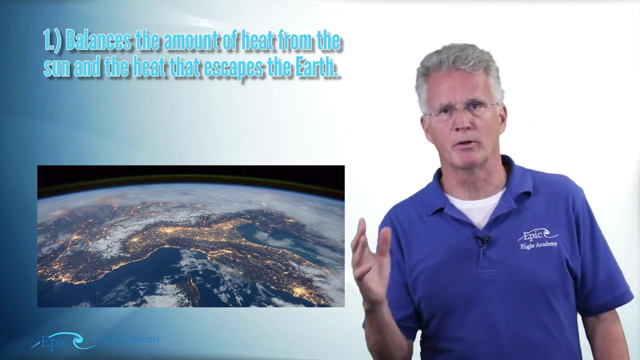 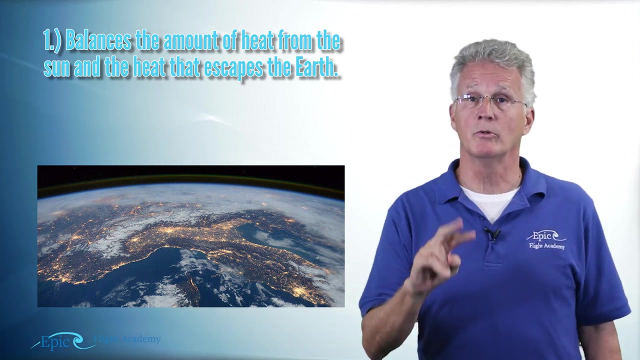 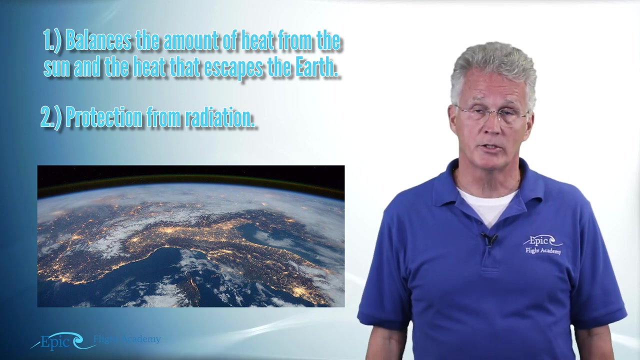 in space. That layer of gases is relatively thin and it serves two critically important functions. Number one: it helps the Earth balance the amount of heat absorbed from the Sun and the heat that escapes from the Earth. Number two, also very importantly, the atmosphere protects us from radiation. 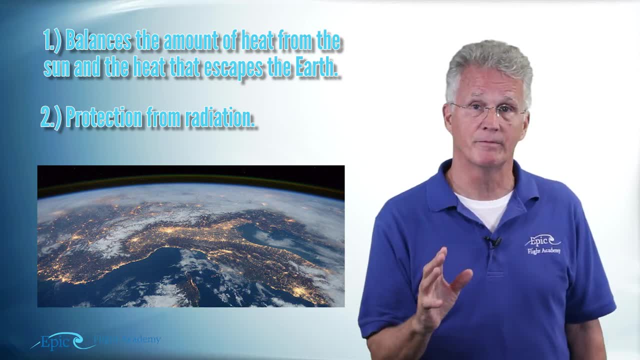 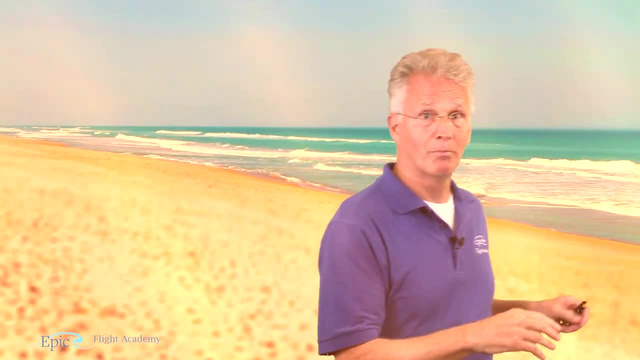 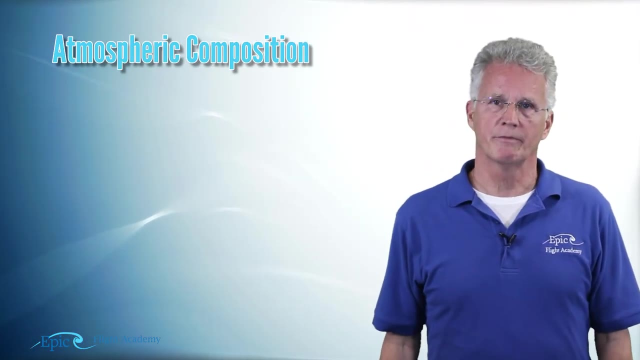 Number three: the atmosphere provides proper protection against hot air and powerful radiation. Number four: in spite of that protection, some of the UV rays still penetrate, and that's what caused me to get a sunburn last weekend at the beach. Now, when we talk about the gas composition of the atmosphere, 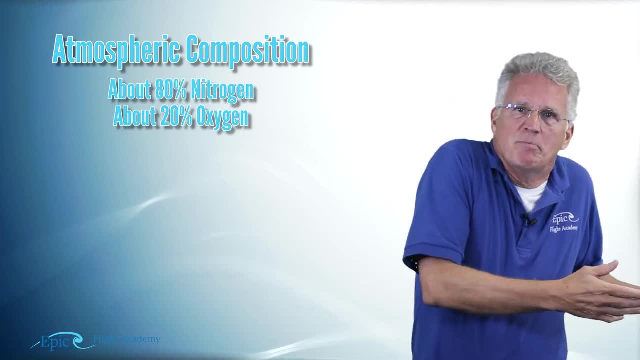 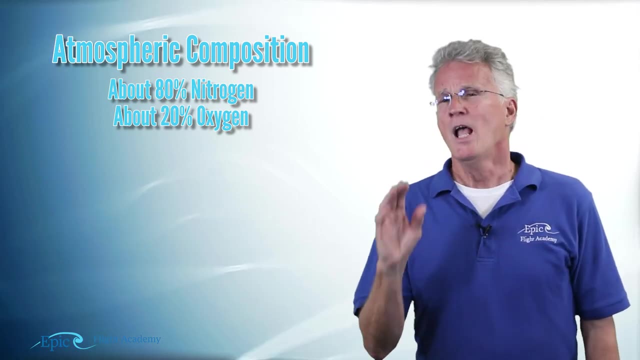 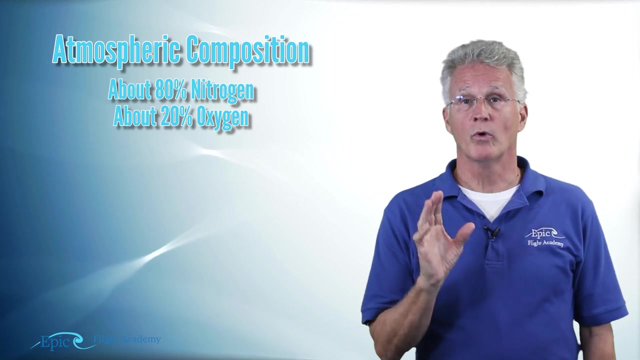 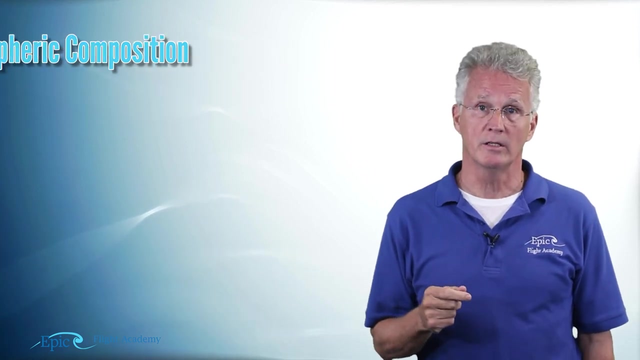 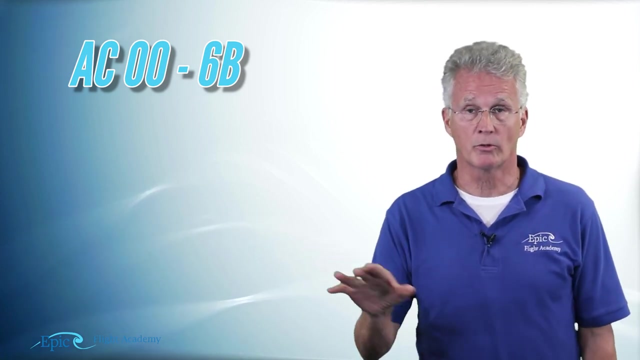 we generally talk about 80 percent nitrogen, 20 percent oxygen. That is approximately true. However, I would like for you to understand more specifically the exact amounts. Our reference for weather will be an FAA Advisory Circular. It is the Advisory Circular 00-6. Bravo, It's a great Advisory Circular. It's been around for. 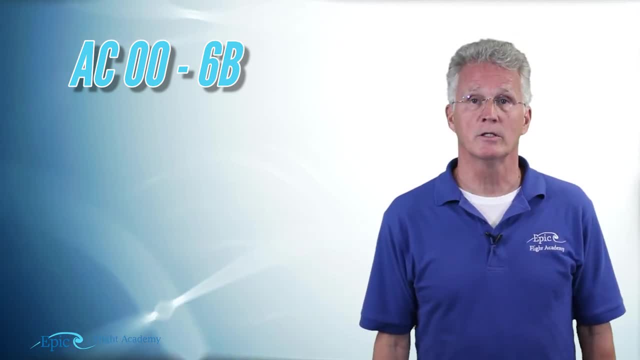 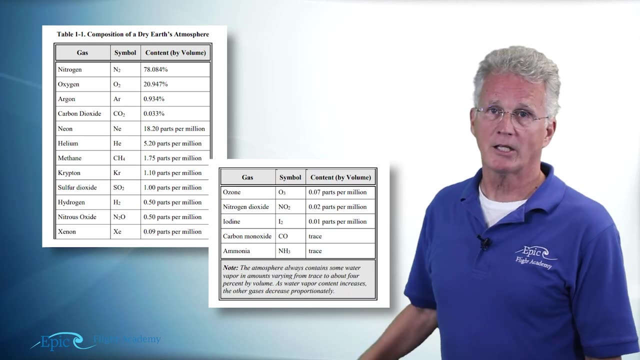 many years, and it's called Aviation Weather. If we look in Chapter 1, we're going to find this table, Table 1-1, and we're going to see much more accurate representations of the gases in the atmosphere. We see, for example, that: 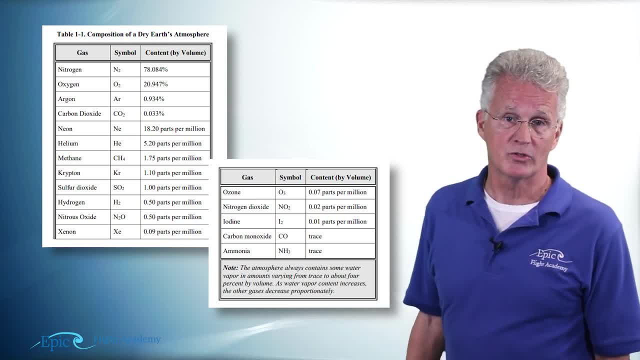 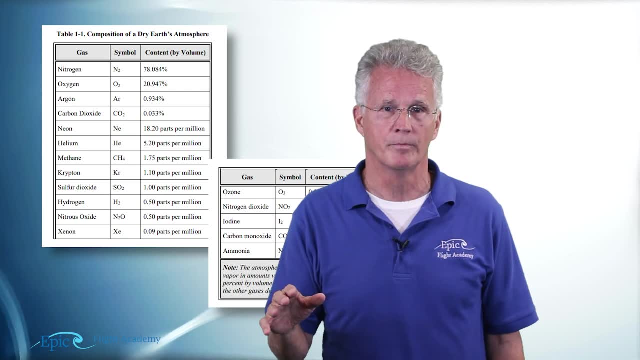 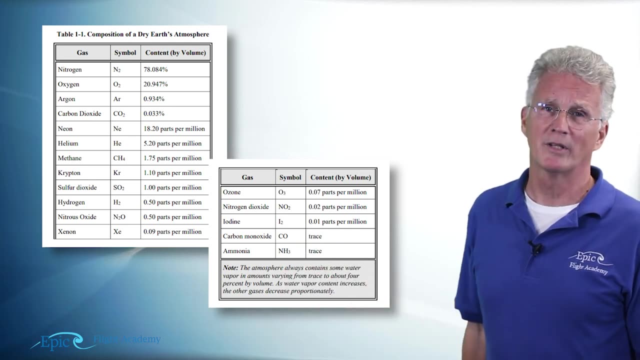 hydrogen is approximately 78.09 percent. we round off the 79, sometime we round it off to 80. Oxygen, we see, is 20.947 percent, and again we round that off to 21,. Sometimes we round it off to 20,, okay. 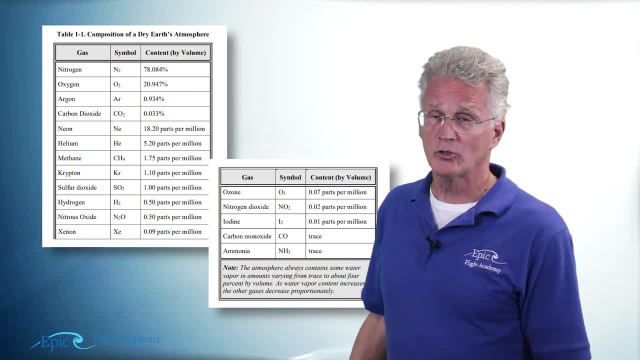 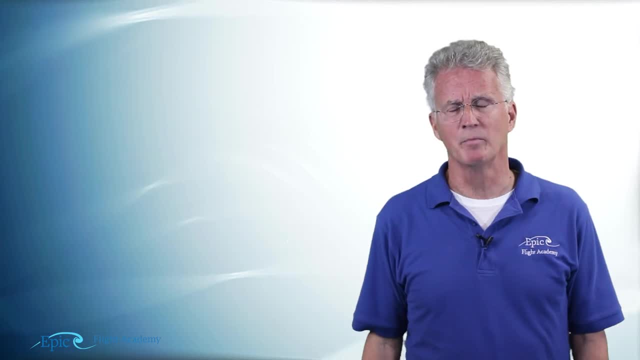 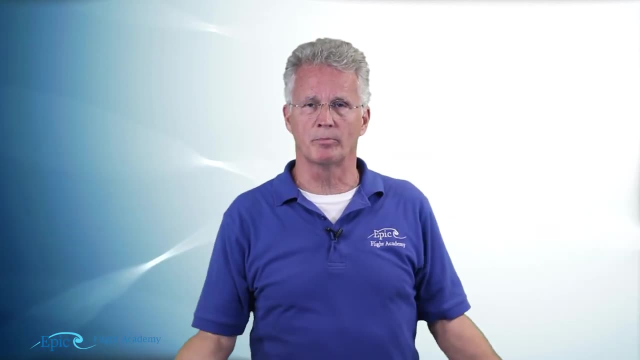 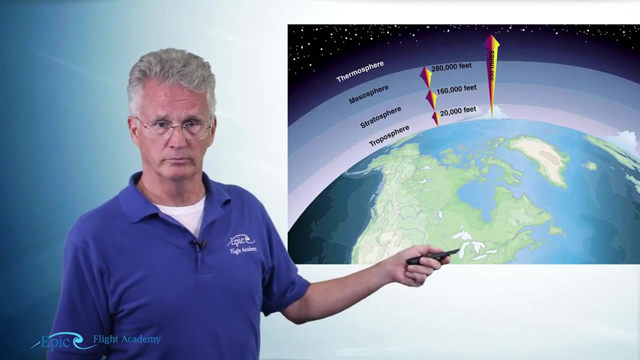 So take a look at the table. You can see all of the actual gases and their approximate, accurate percentages. Now the atmosphere has layers throughout it as it surrounds our planet. This graphic you're going to see in EPIC's online Schoology course. 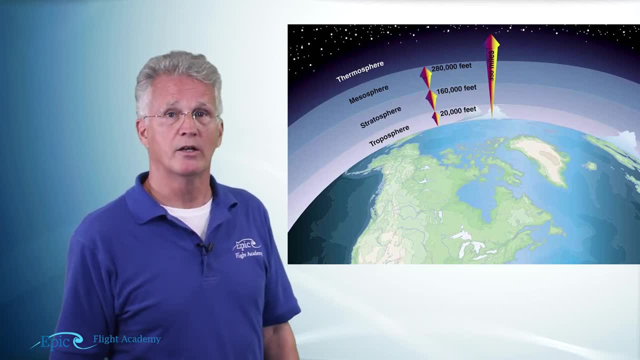 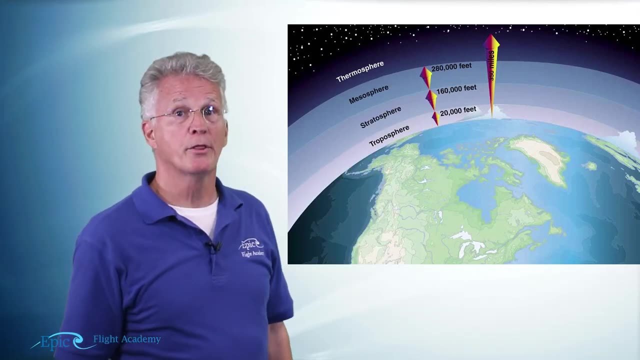 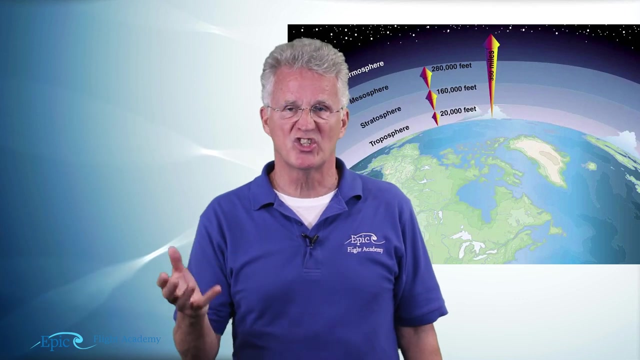 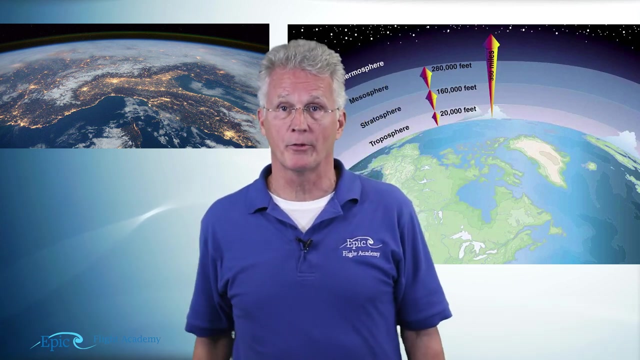 Now notice it shows us four layers and notice that those layers are represented as being much thicker than they actually are in reality. They're represented thicker so that we can see them and study them. Go back to the photograph from space to see in reality how thin the atmosphere. 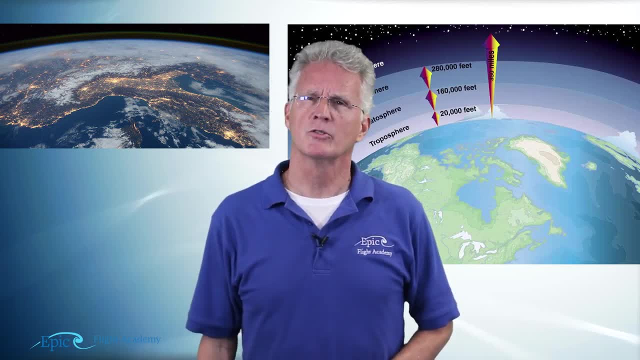 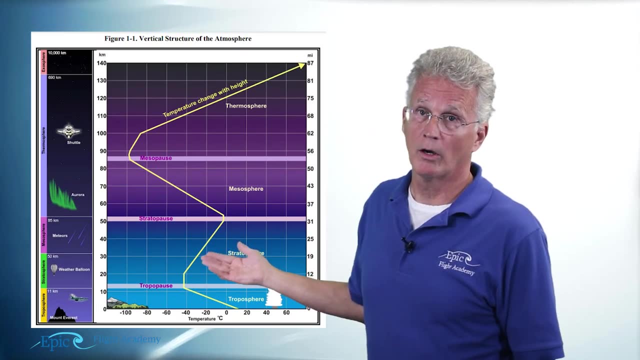 actually is compared to the whole planet. So let's take a look at these layers. How many are there? Well, in this graphic again, where are we? Aviation weather 006B, chapter one We're showing the first layer is the troposphere. In that first layer the vast majority of weather occurs. Then we reach the tropopause at approximately six to seven miles, or 13 to 15 kilometers. You see miles on the right-hand side of the chart and kilometers on the left. Well, how many feet is that? 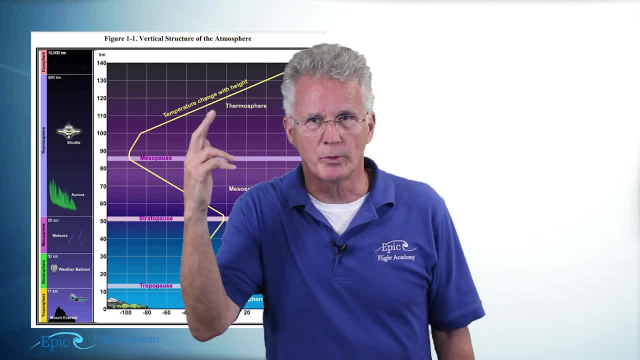 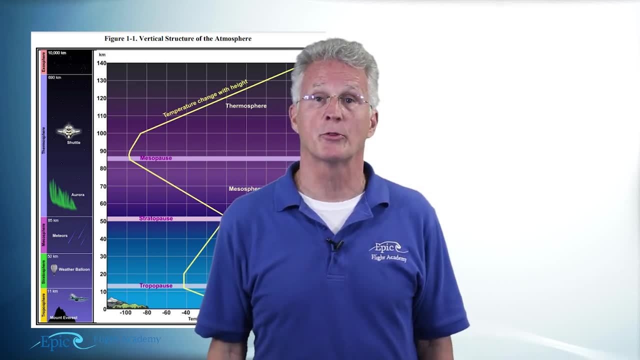 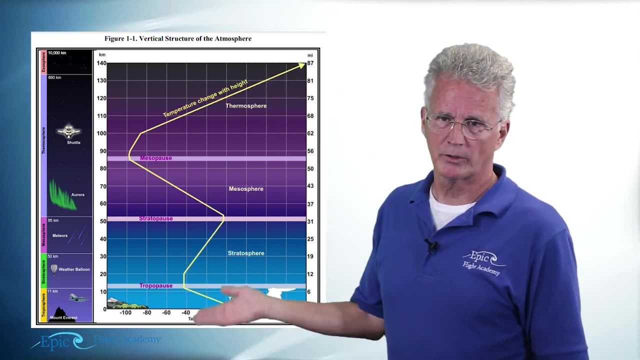 Because, as pilots, we think of altimeters and we think in terms of feet. A quick conversion for you: A kilometer is 3,280 feet. So above the tropopause we get to the stratosphere, Then the mesosphere. 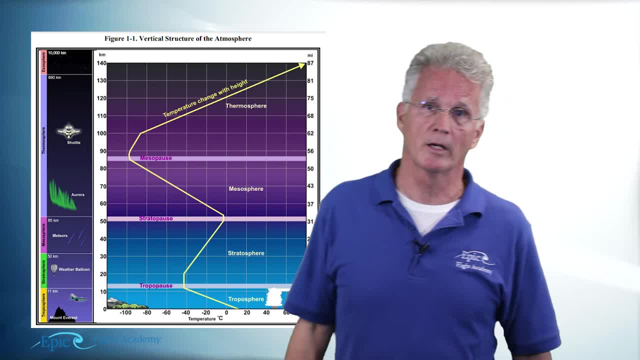 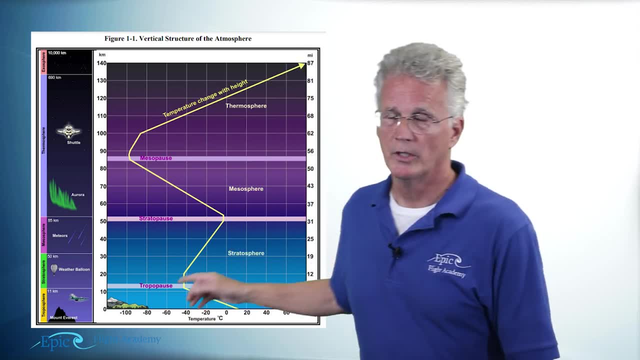 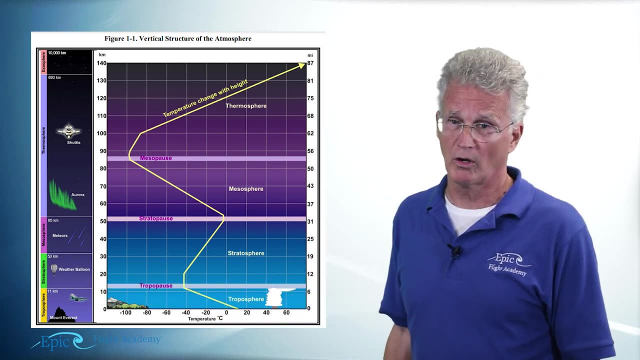 Mesosphere and the thermosphere. So how many layers in the atmosphere? You got it. There's four layers. Now, on this graphic, I'd like you to notice this yellow line. This yellow line is showing the temperature and you can see temperature in Celsius across the bottom. 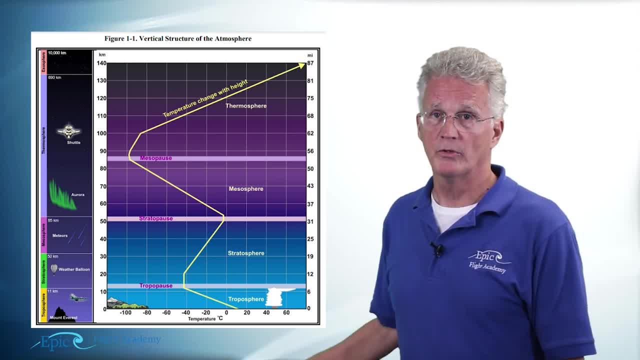 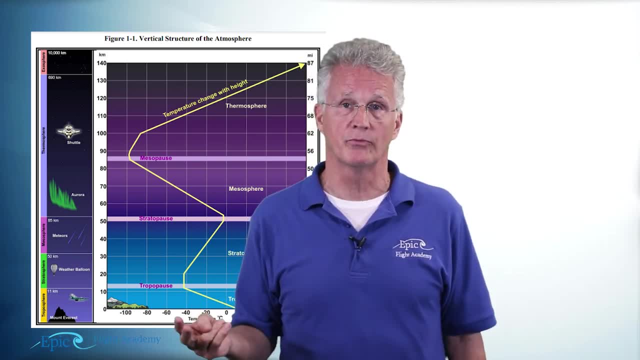 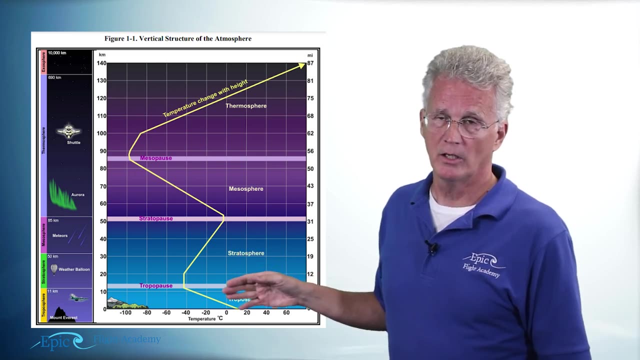 Notice, as we go up into the troposphere, the temperature goes down. Now our flight instructor probably told us that the average is two degrees per thousand feet, Two degrees Celsius per thousand feet. But an interesting thing happens at the tropopause As I continue higher in the stratosphere. notice the temperature actually goes up. Well, why is that, Folks? the reason for that is ozone. Ozone absorbs that harmful radiation that we mentioned earlier And that causes the temperature to rise. Then we get out to the mesosphere. 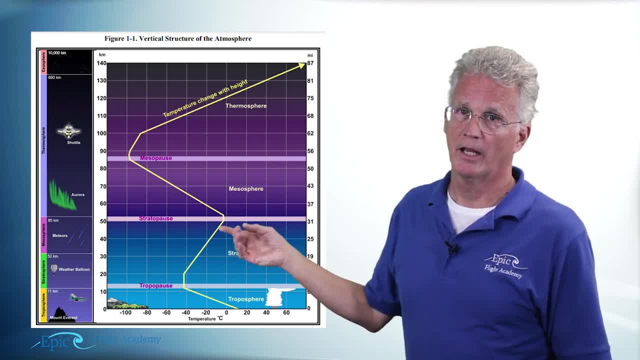 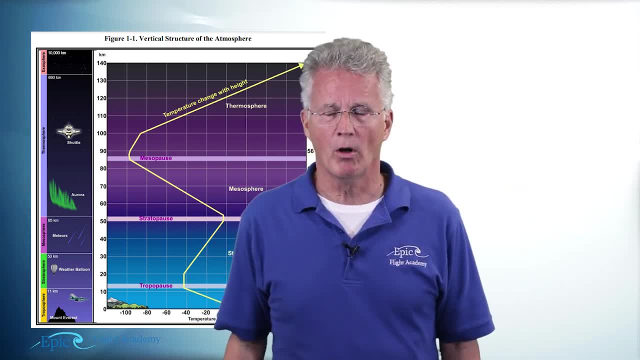 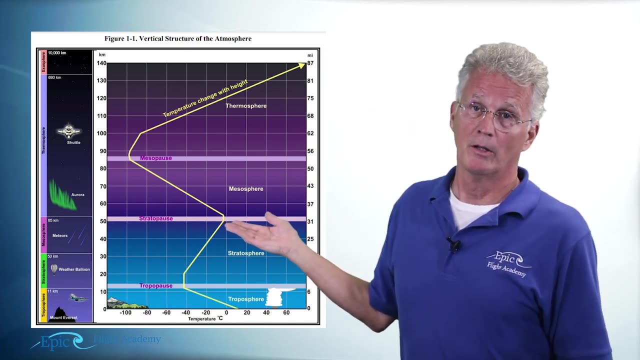 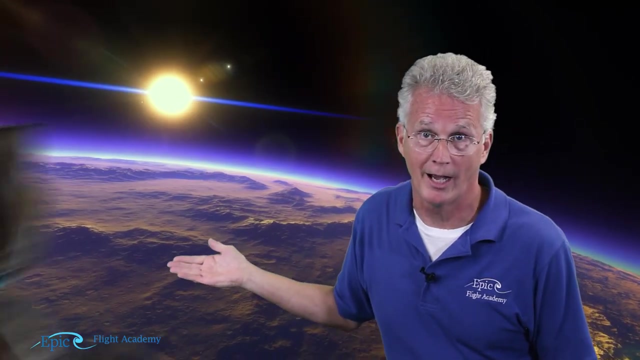 where we have very little atmosphere left and we see the temperature again starting to drop. And then we get to the mesopause and into the thermosphere. And now we're out at altitudes where ATC might say traffic advisory space shuttle at 2 o'clock.